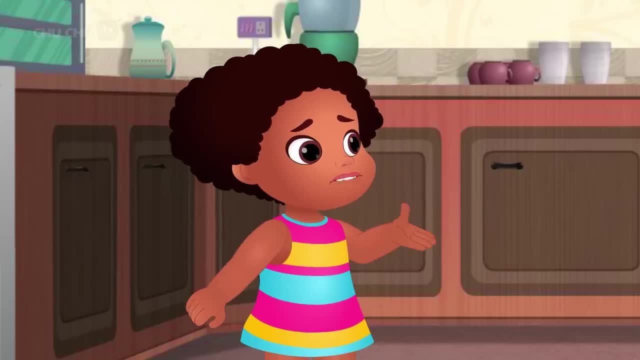 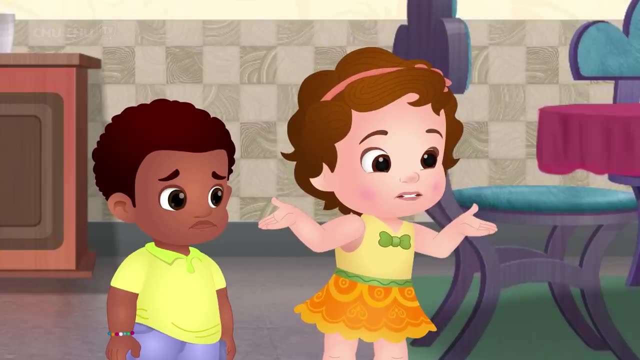 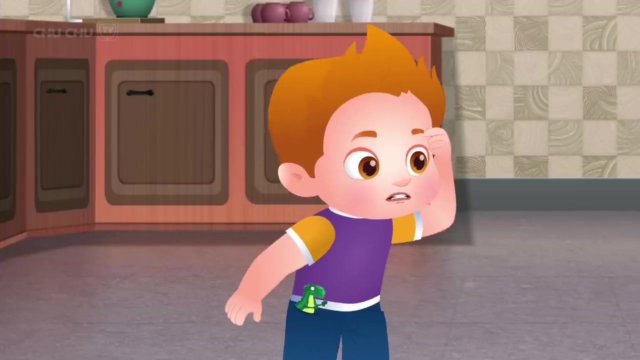 Eww, Custly, please, don't eat with your mouth open. It's disgusting, And don't make those sounds while chewing. Custly, Please, Please, Oh, please, Please, Please, Custly, please, Custly, please. 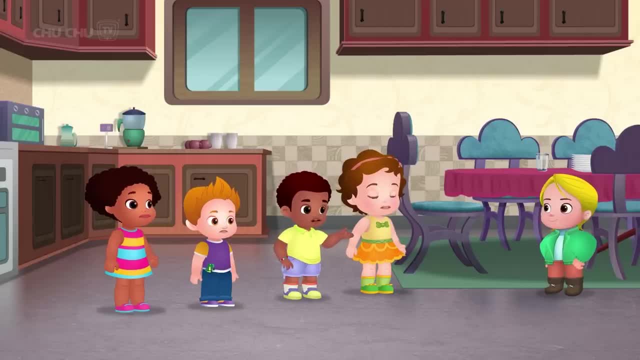 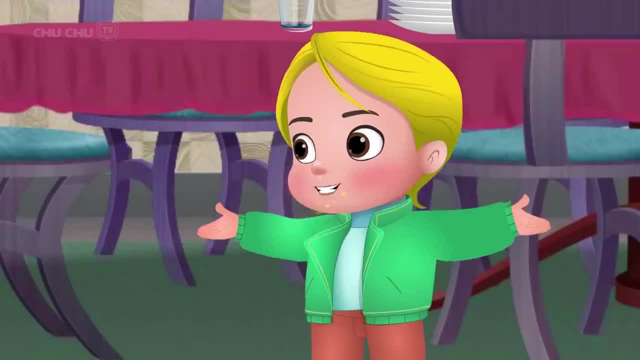 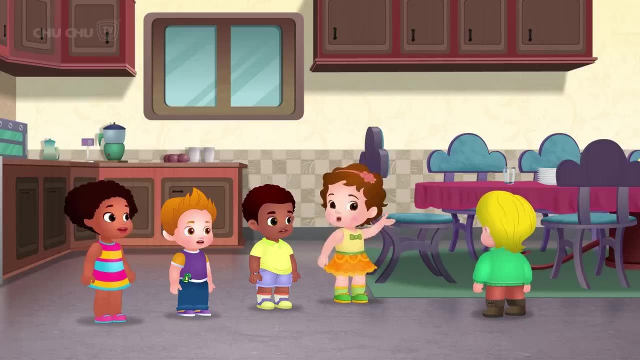 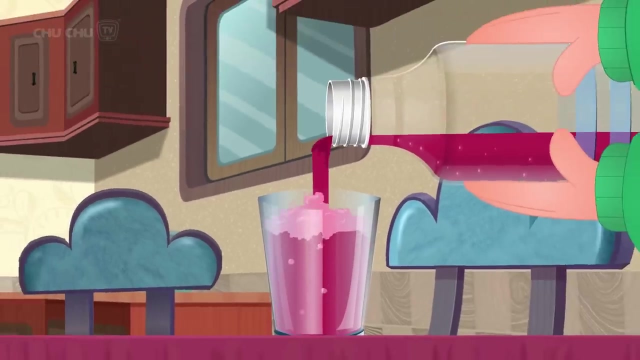 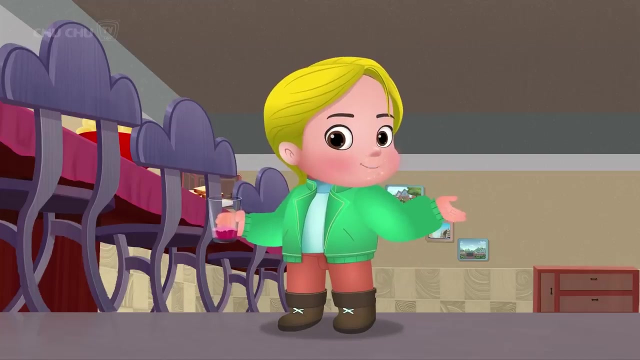 Hey, What's your problem? I enjoy eating this way, But people around you don't enjoy watching you. Yeah, it grosses them out. That's just too bad for them. Yummy, You know what I like best about soda? 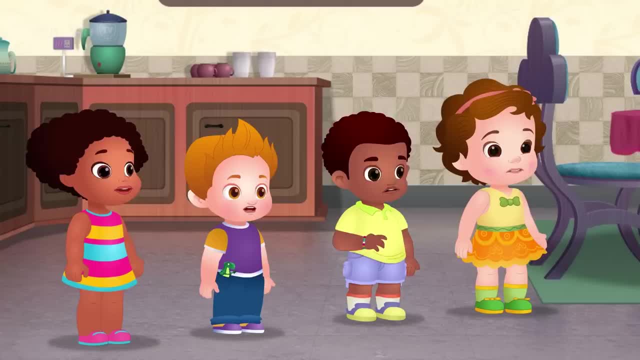 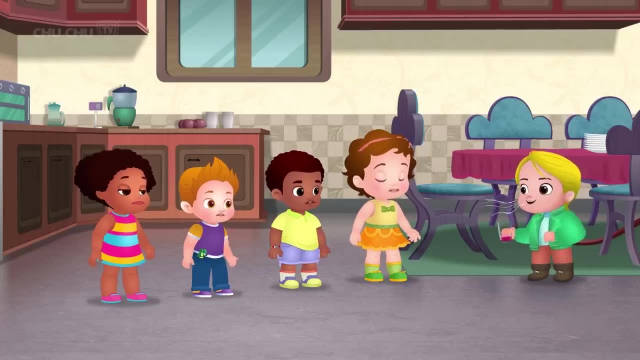 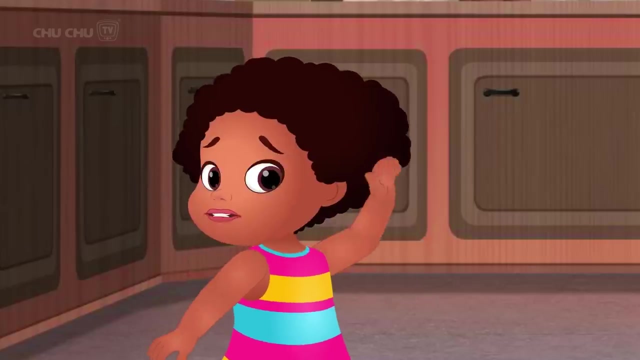 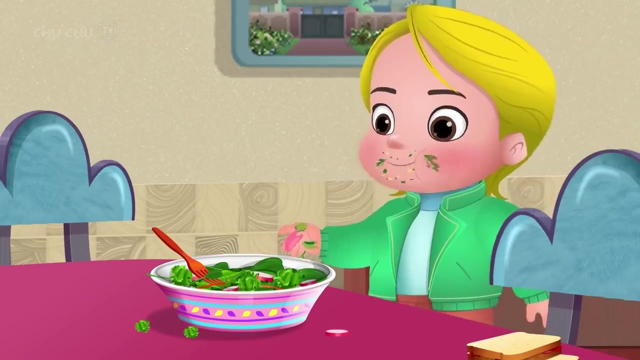 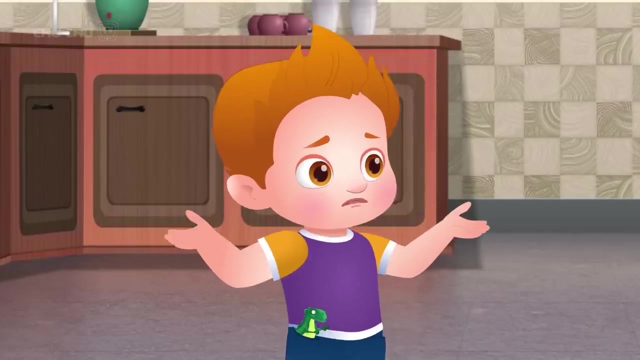 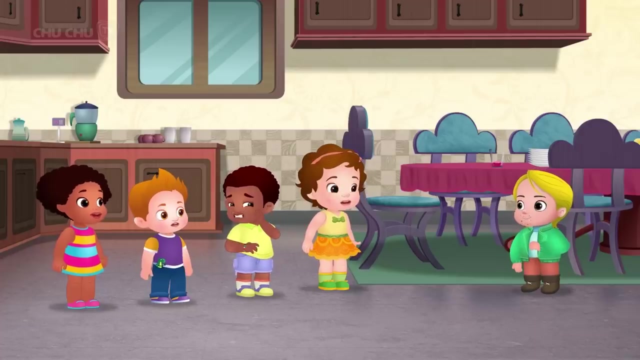 The burps Custly. That's really bad manners, But it's so much fun. Ah, Bad manners weren't funny. Custly Gosh, what a mess you make while eating. Custly, That's not polite. There's food all over your face. It's disgusting. 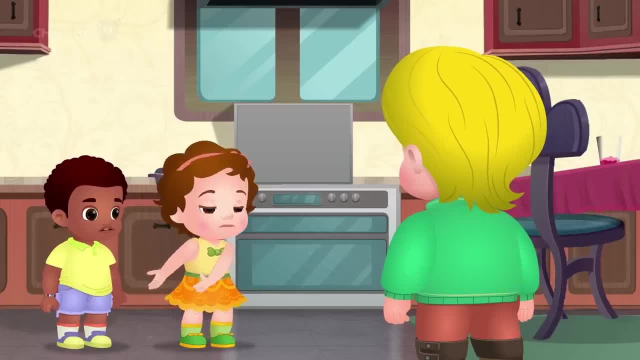 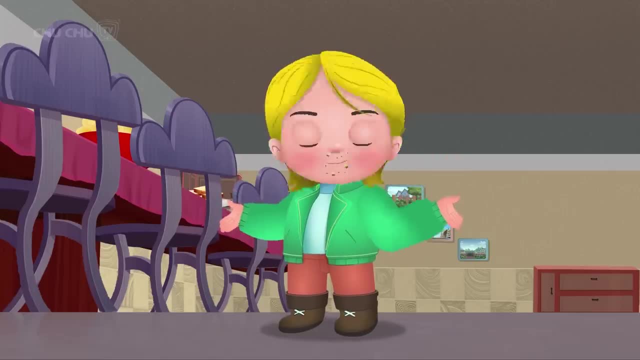 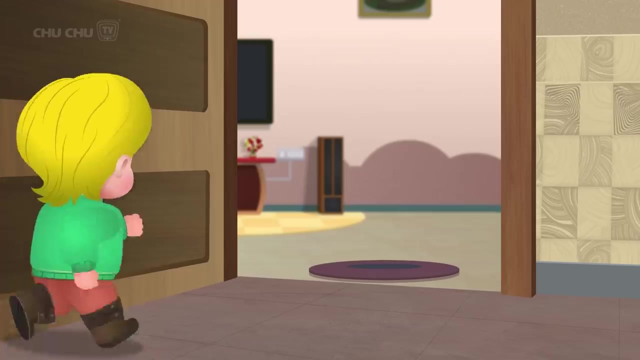 Yeah, I'd hate to be sitting next to someone with such terrible table manners. Well then, don't Your problem. I'm headed to the yard to see if the mommies and daddies are on their way, Custly's being so gross. 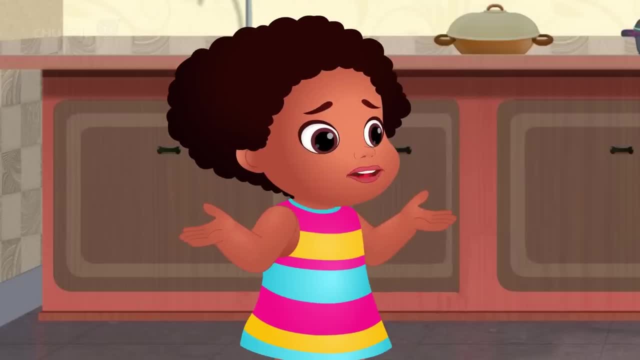 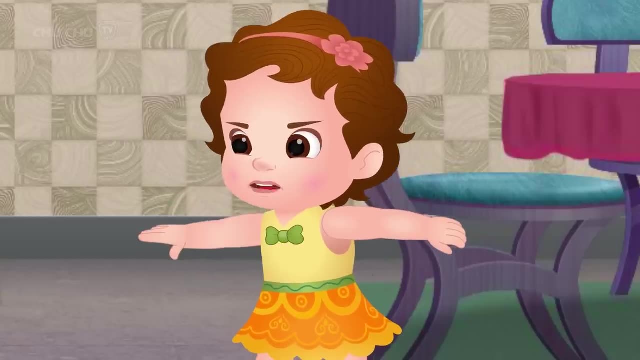 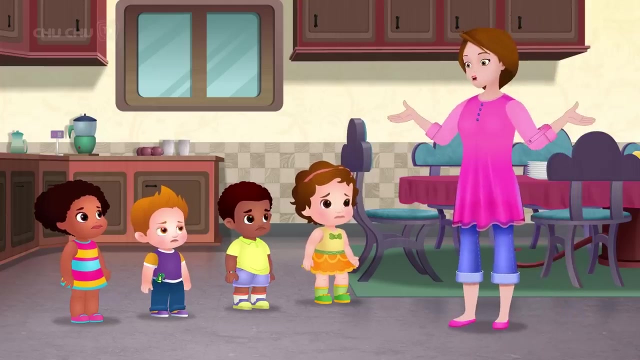 If he behaves like this during the party, all the parents will be disgusted. Oh no, We can't let that happen. It's better to call off the party. What's up kids? Why does everyone look so sad? I thought you'd all be excited about your mommies and daddies' party. 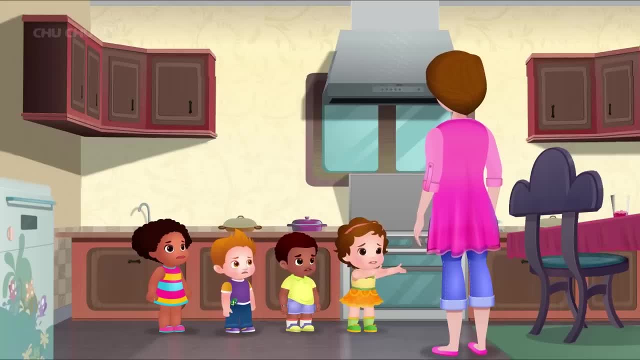 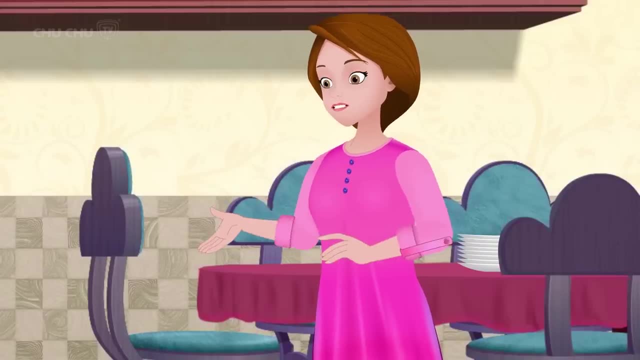 Mommy, we were really excited about this party, But not anymore. We want to call it off. Why? What happened, darlings? Tell me, Maybe I can help fix things. Mommy Hesley's doing disgusting things. 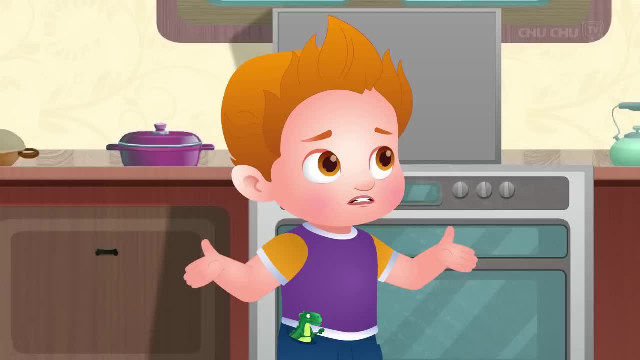 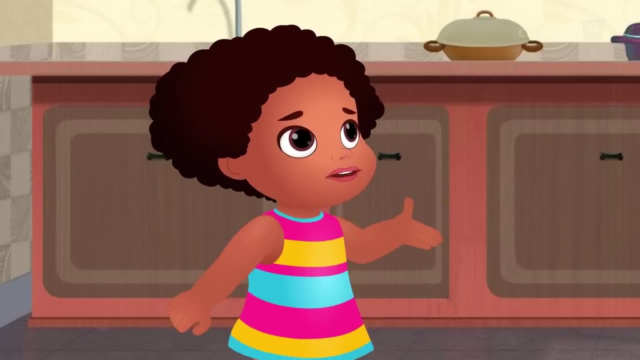 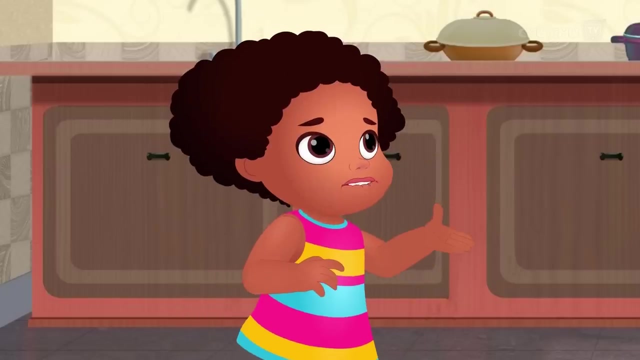 He's eating with his mouth open and burping And spilling, And he won't stop Because he thinks it's funny. Yes, Mrs Charlie Custly's terrible table manners will gross out all our parents. That's why we want to call off the party. 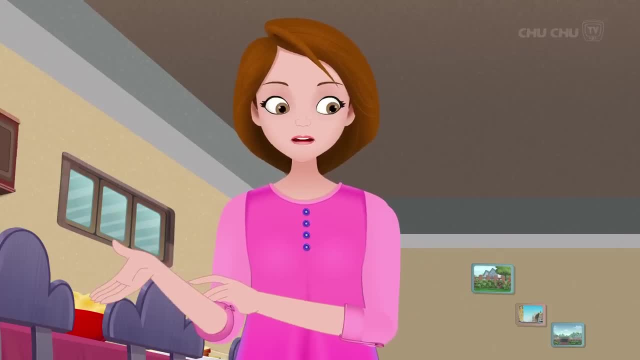 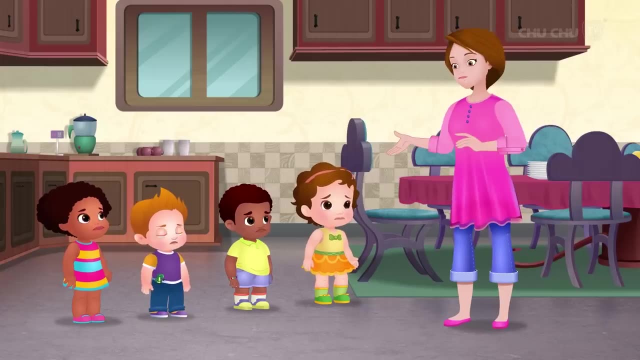 Hmm, That doesn't sound very pleasant at all. But you know what kids. You're his best friends And if you want to do what's good for him, You must help him improve His table manners. But how, Mommy? 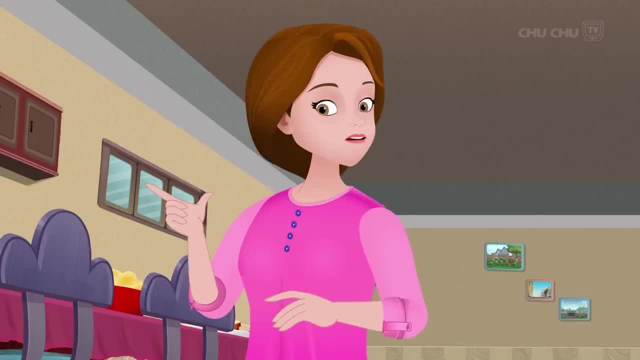 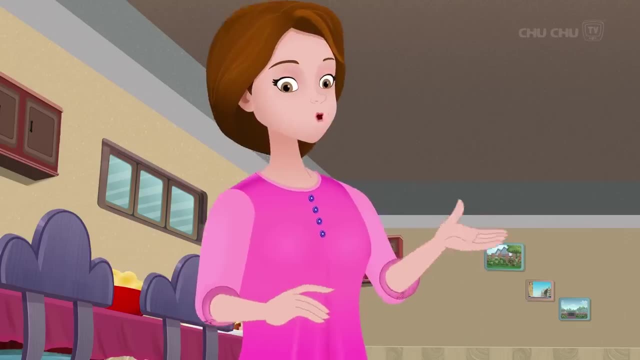 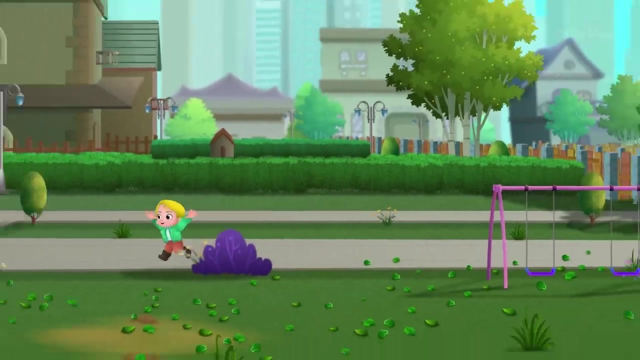 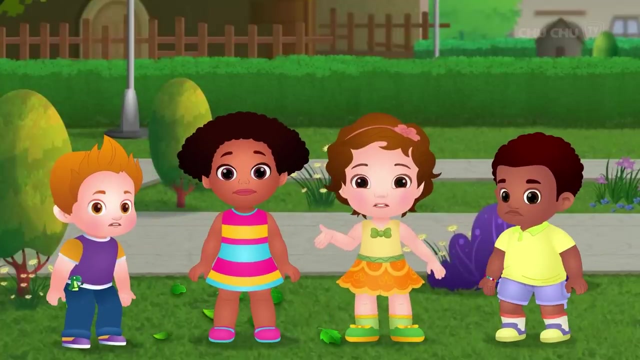 He just laughs at us. So here's an idea: Instead of canceling the party for everyone, You need to tell Custly that he's not welcome to the party If he shows such bad manners. That's a great idea. Custly, we need to talk to you. 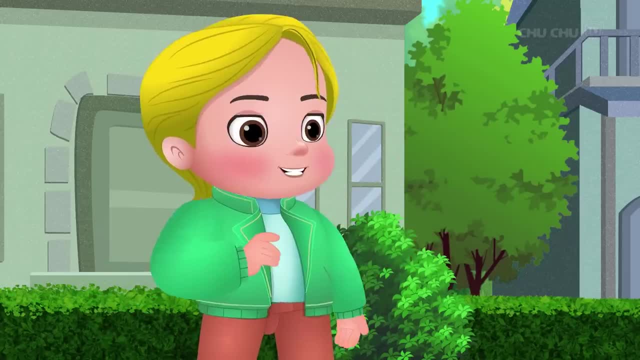 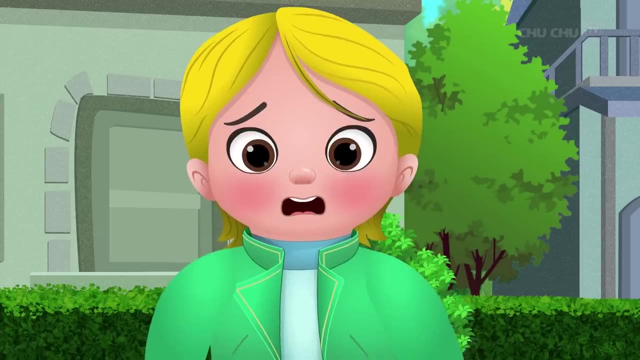 If it's about the way I eat, I'm not listening. You're gonna have to put up with it. No, We're not gonna put up with it. Huh, What does that mean? That means you're not invited to the Mommy's and Daddy's party. 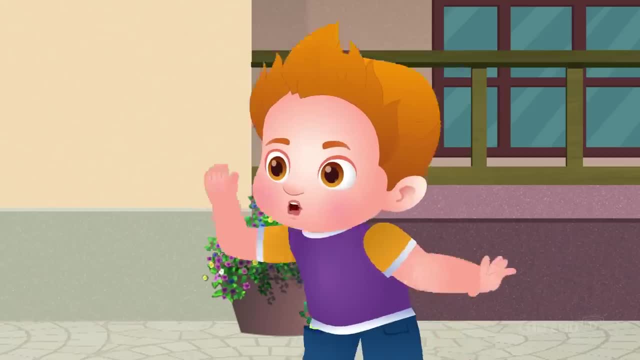 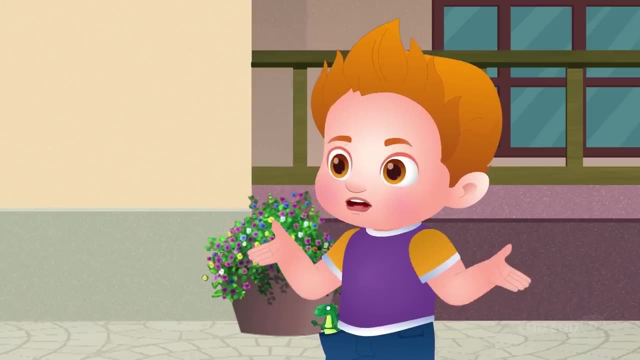 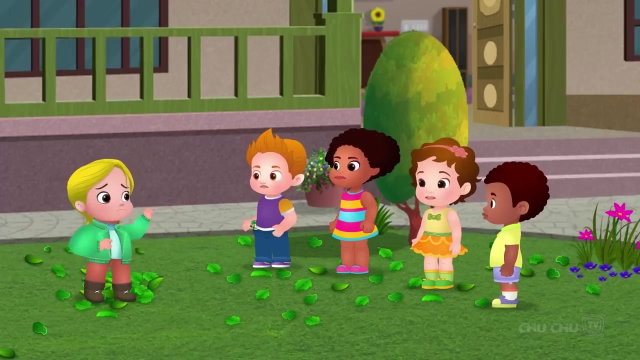 What, But why? Because your bad manners will ruin the party for everyone. That's why we can't have you at the party. My Mommy said. You said so too. Your Mommy said that: Okay, listen, I really want to be at the party. 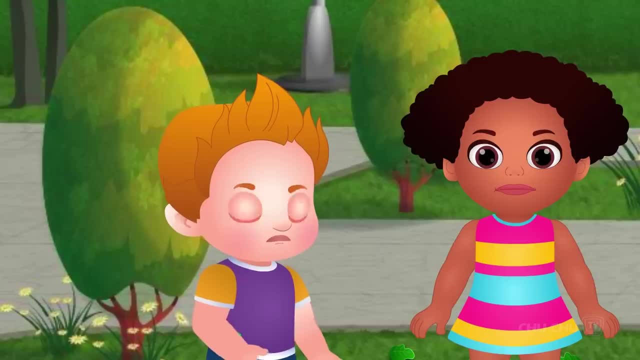 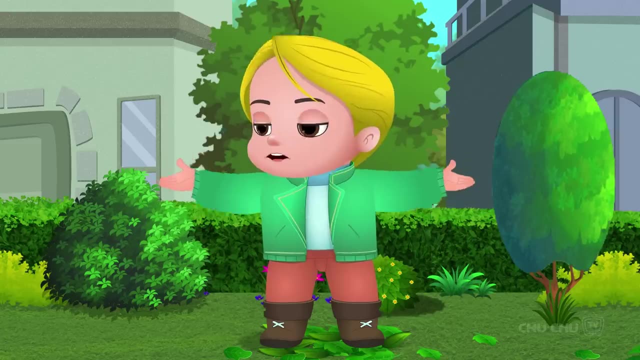 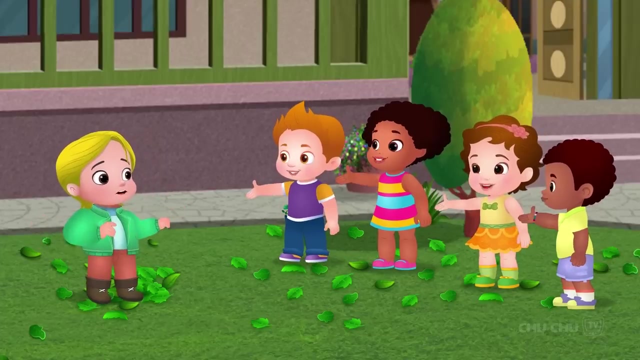 I promise I'll be well-mannered. I'm sorry, I won't behave like that anymore. Please, please, please, let me attend the party. I won't be gross anymore, You promise, I promise. Okay, we'll give you a chance, Custly. 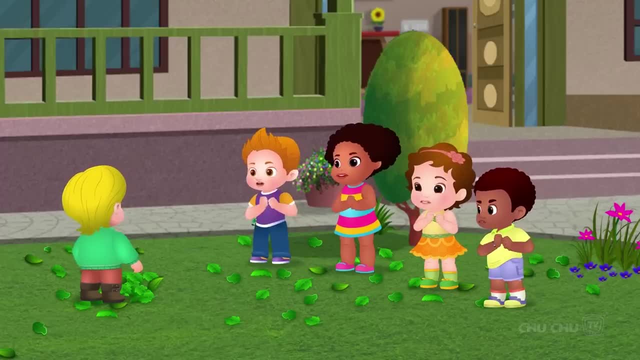 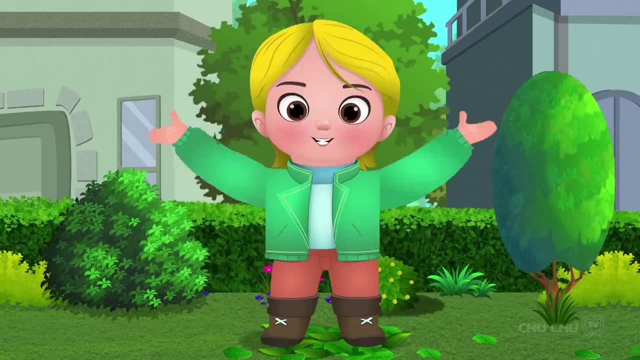 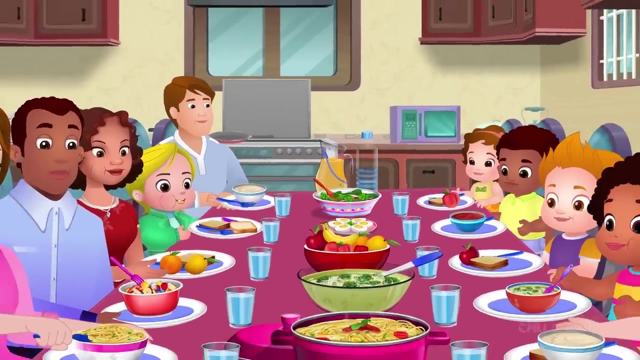 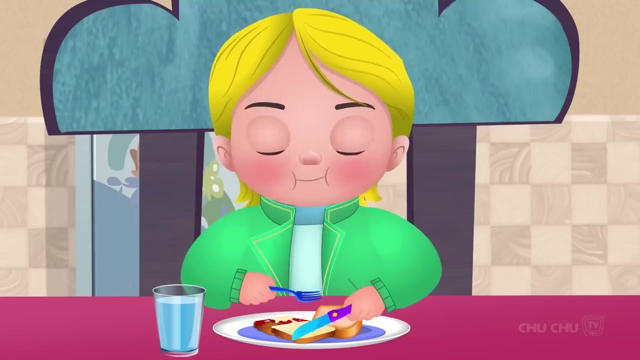 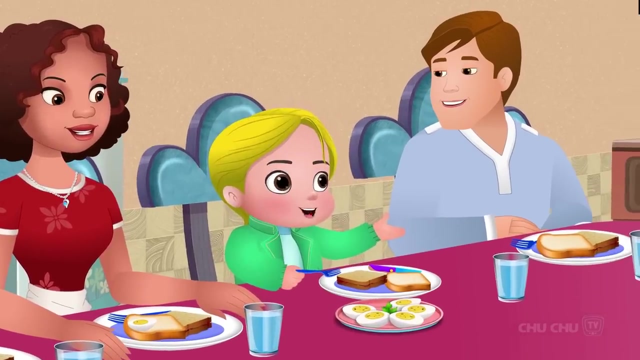 But if you're ill-mannered again We won't be your friends. You know who's gonna be the best-behaved kid at that party. Super adorable me. Please have some. Mrs Williams, May I serve you one, Mr Charlie. 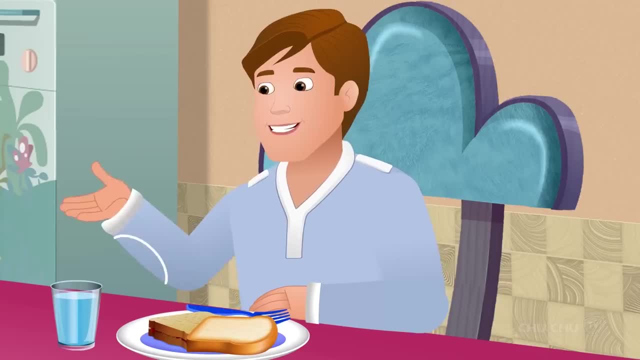 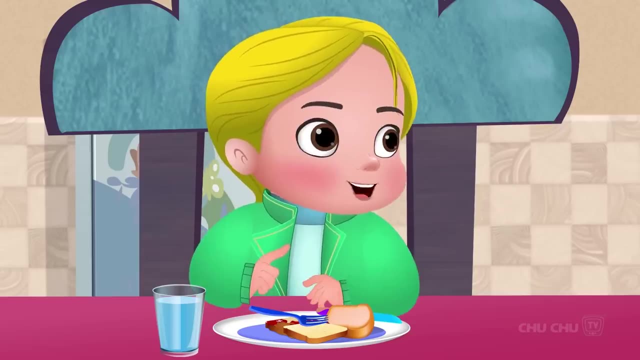 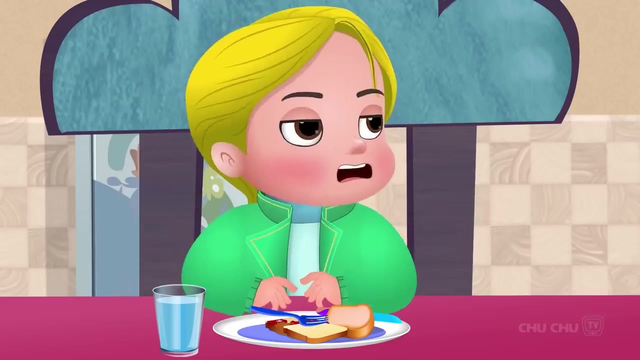 You're a very polite kid, Custly. Yes, you have excellent table manners. Thank you, Mrs Williams and Mr Charlie. Actually, I get that a lot. I'm so bored of being praised all the time. Oh, Watch me have some fun. 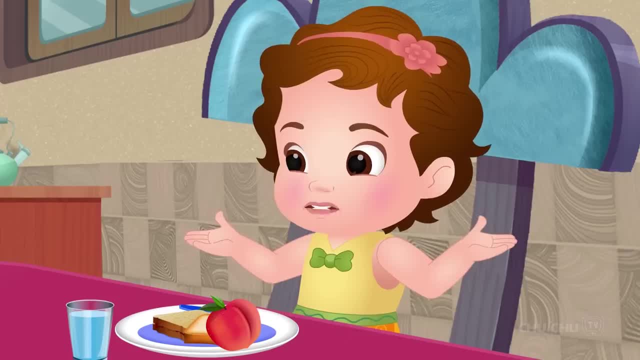 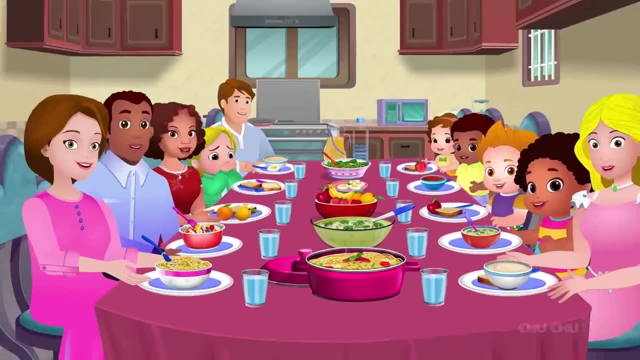 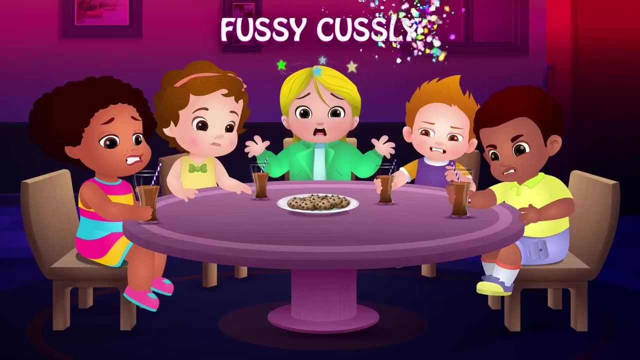 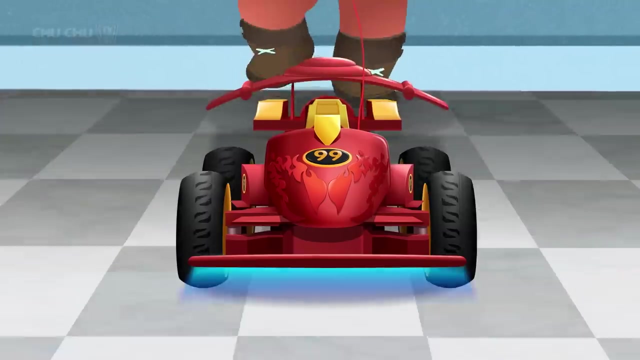 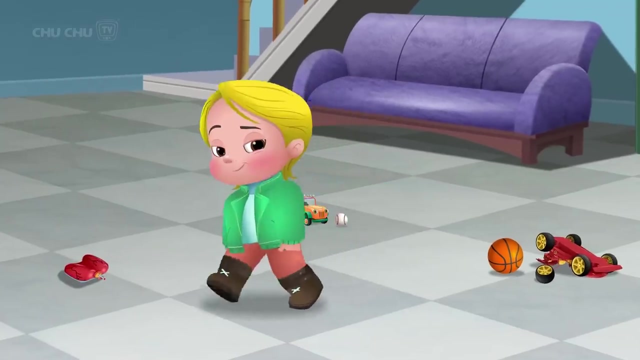 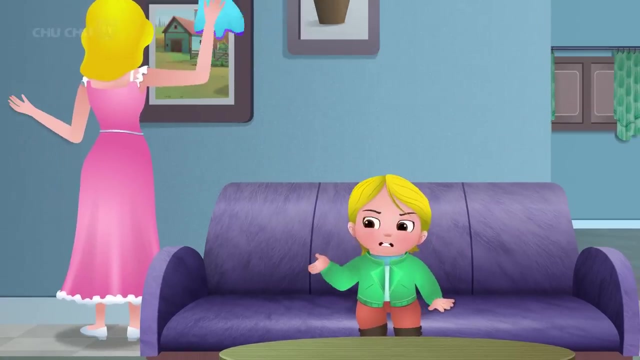 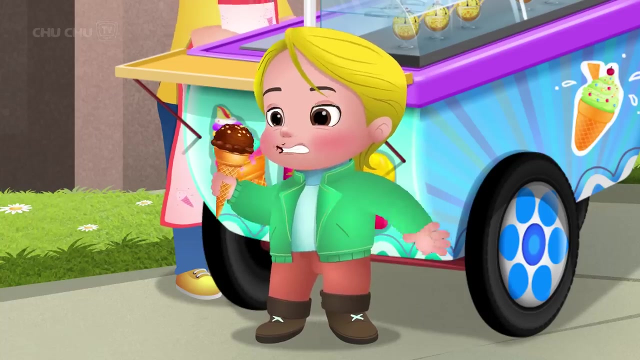 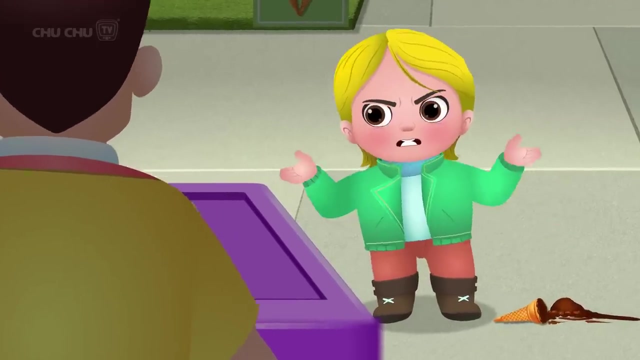 Where are your manners, Custly? Don't you know? you're supposed to cover your mouth while yawning? Custly was a fussy little boy. He always complained about everything. Oh, This cushion isn't soft enough. Ew, I don't like this ice cream. 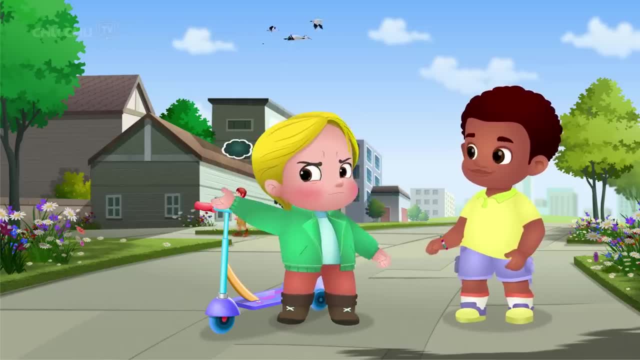 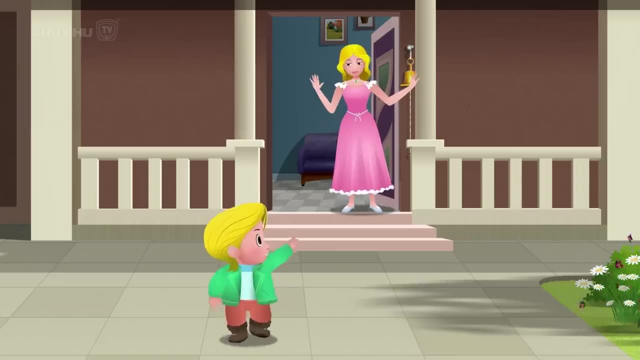 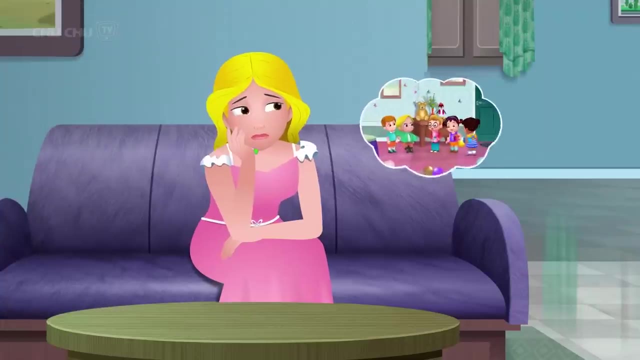 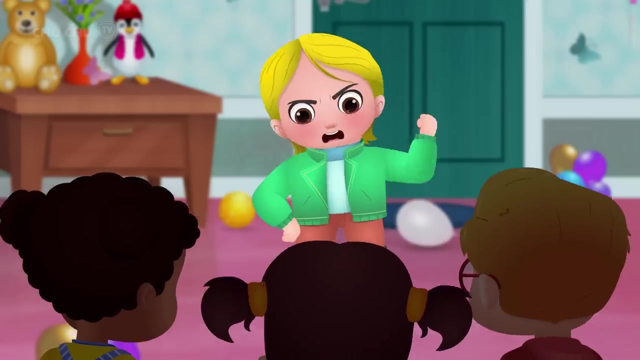 Chica, the gift you gave me isn't nice at all. Huh, Custly's mother was quite worried about him. Custly grumbles and fusses about everything. He is very rude. He must learn how it makes others feel when he complains like that. 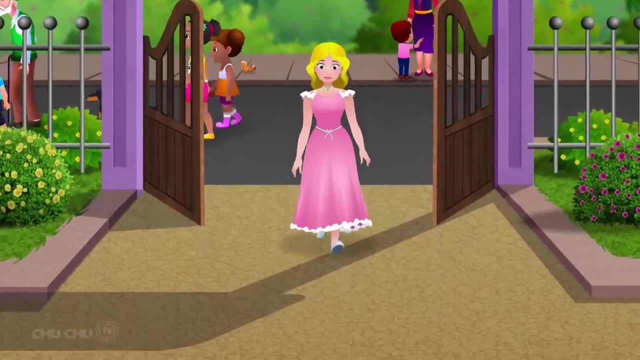 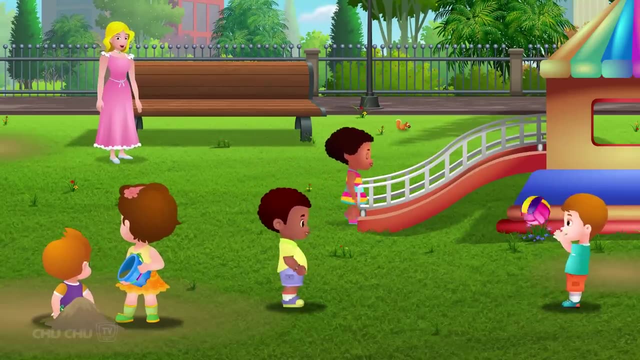 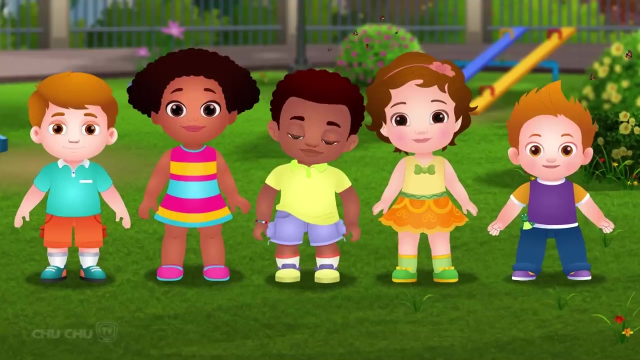 Custly's mother doesn't want to be a burden to him. One day, Custly's mother came up with an idea. She spoke to Choo-Choo and Custly's other friends: I need your help, children. Custly's mother then asked Custly to invite his friends home. 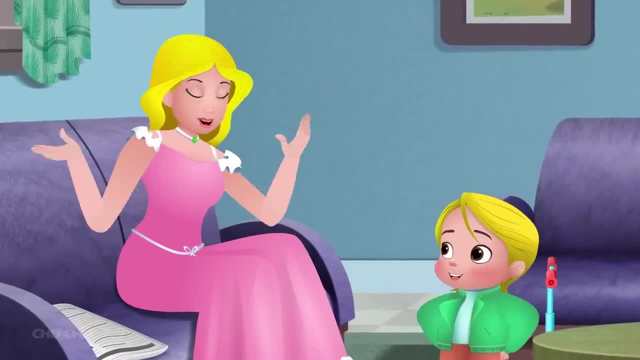 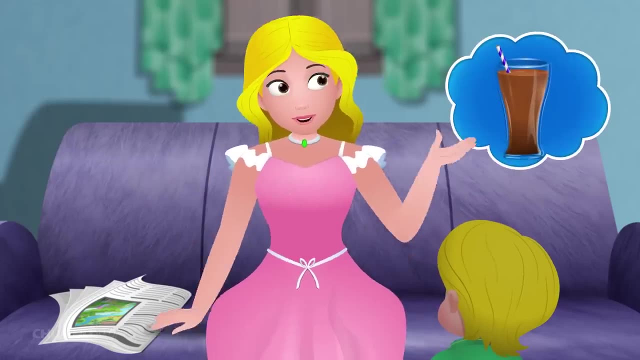 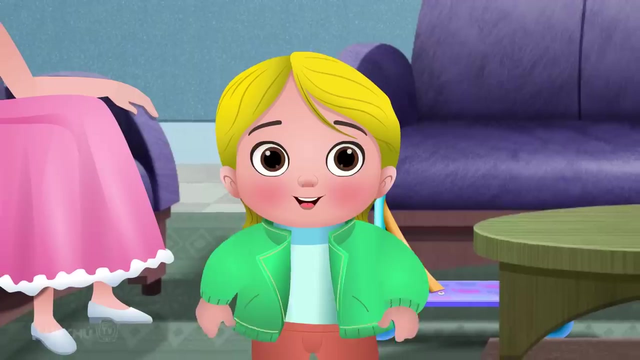 Custly, Why don't you invite your friends over today? Tomorrow, You can all play together. I'll help you bake cookies and make chocolate milkshakes. Good idea. Mom Custly liked the idea, And so he invited all his friends. 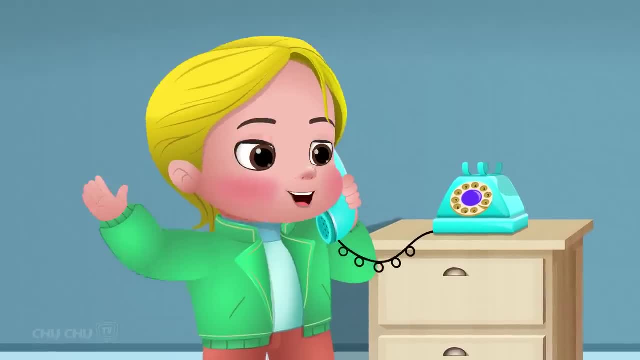 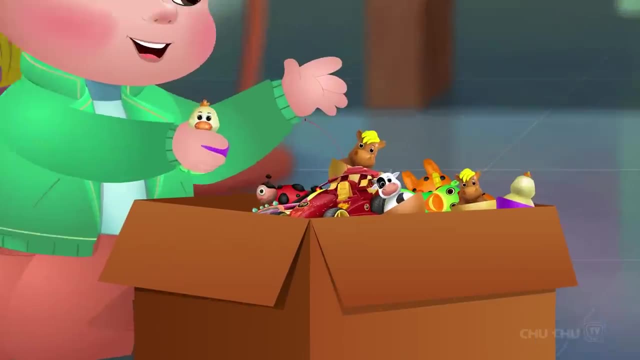 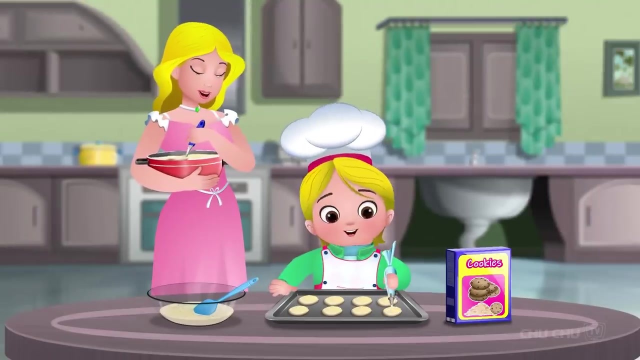 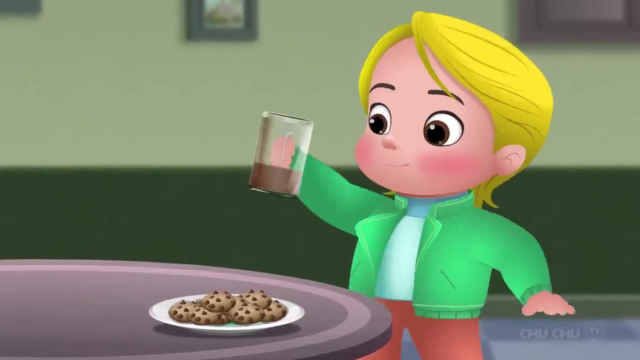 Please come over tomorrow, We'll have lots of fun. The next morning, Custly took out all of his favorite toys and games. We're going to have fun playing with these things. He then baked cookies and made chocolate milkshakes- Mmmmm. 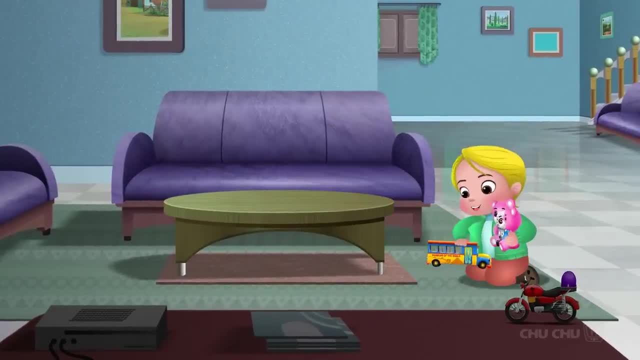 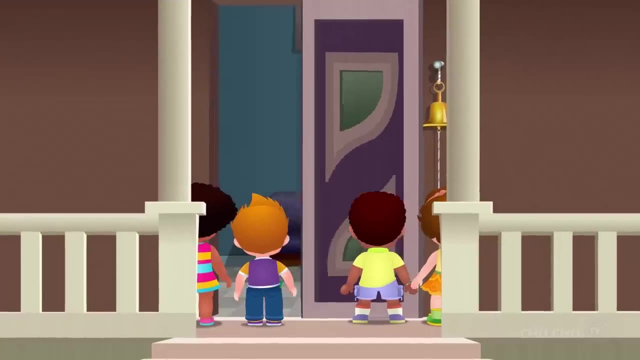 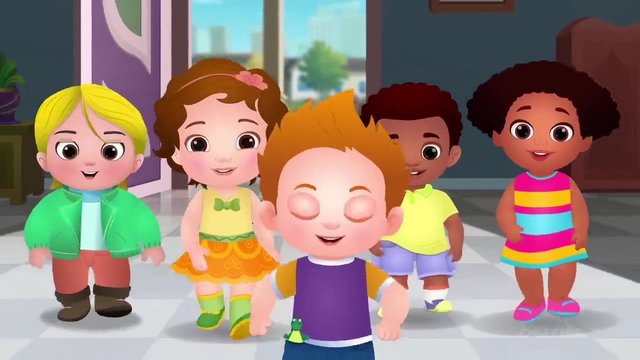 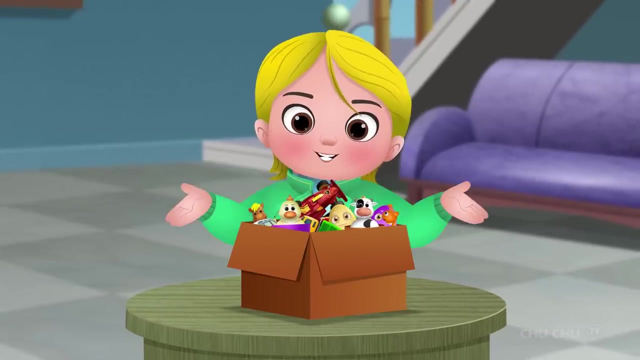 Custly then made the living room very comfortable for his friends. Soon Custly's friends came by. Hi Custly, Hi everyone, Come on, Let's play. Custly brought his toys and games out. These are my favorite toys and games. 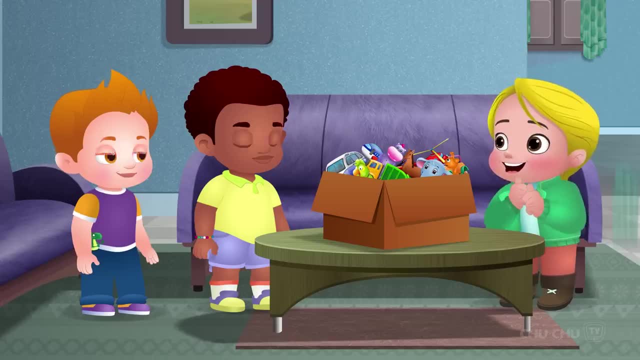 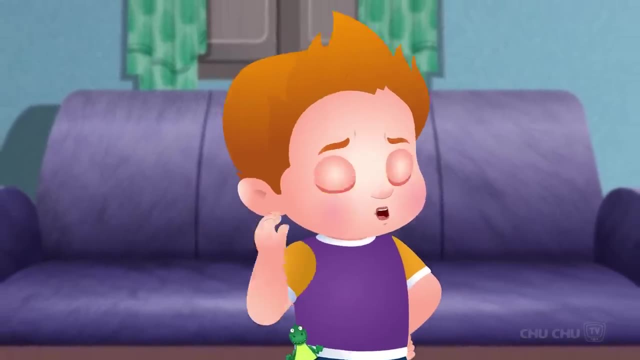 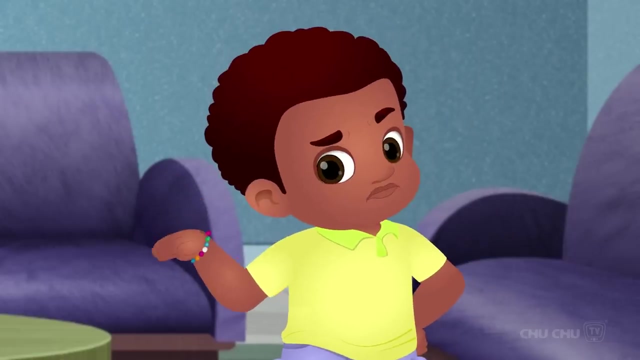 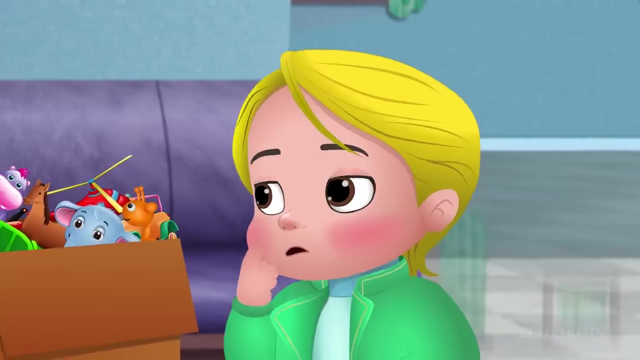 Let's play with them. But Chacha and Chica made a fuss. I don't want to play indoors, Custly, I want to go out. Huh, I don't like your toys and games games, They are boring. Huh. Custly didn't know what to do. He felt like Chacha and Chica. 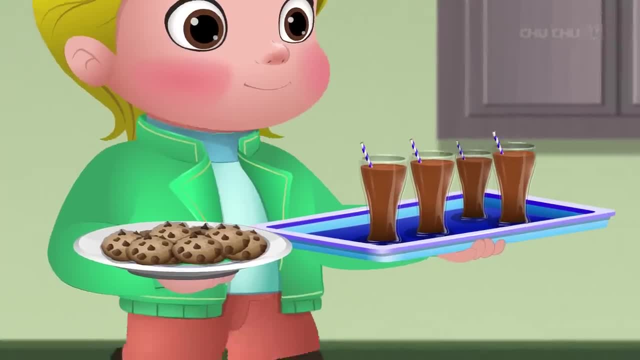 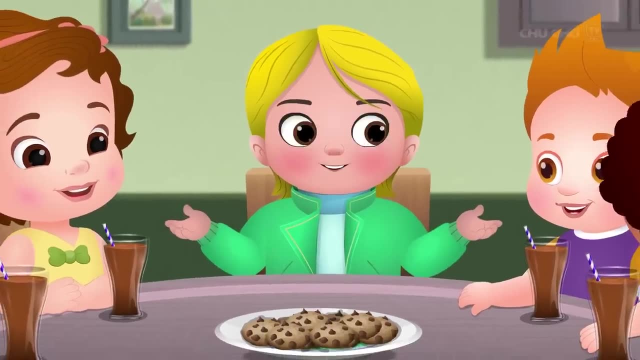 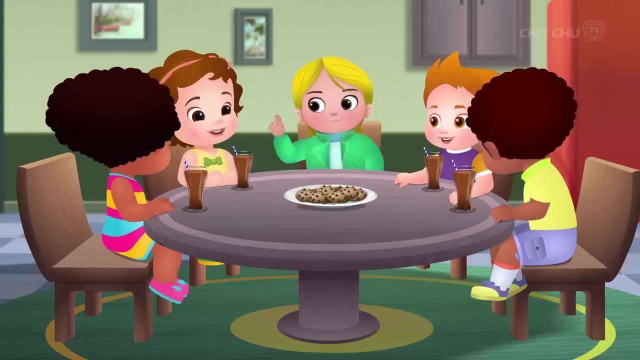 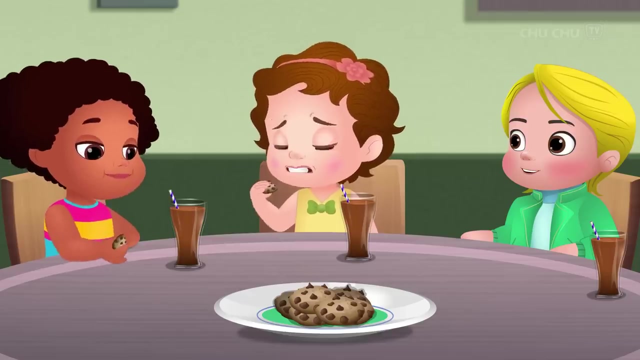 were being very fussy. Custly then brought out the cookies and milkshakes he had made Everyone. I've baked cookies and made chocolate milkshakes for all of us. I hope you like them. Everyone took a cookie and a milkshake But to Custly's surprise, they all started. 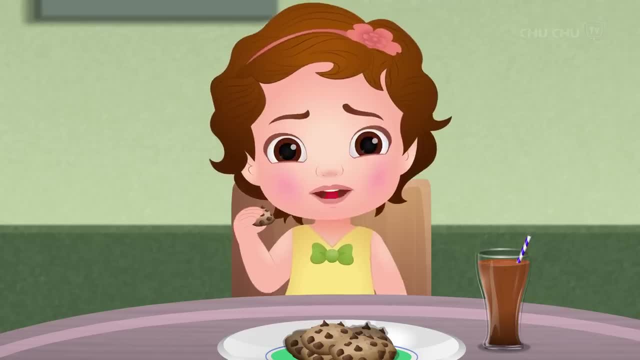 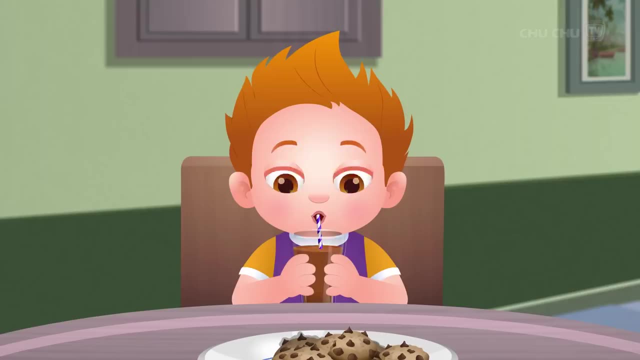 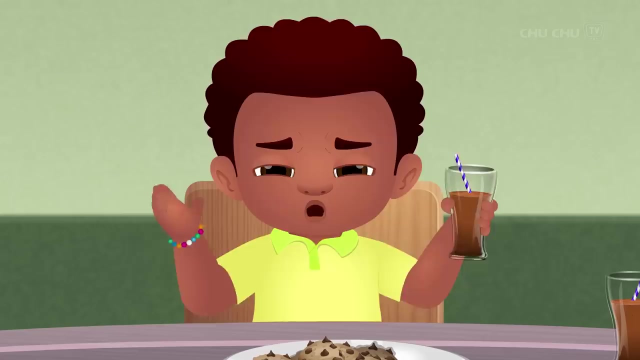 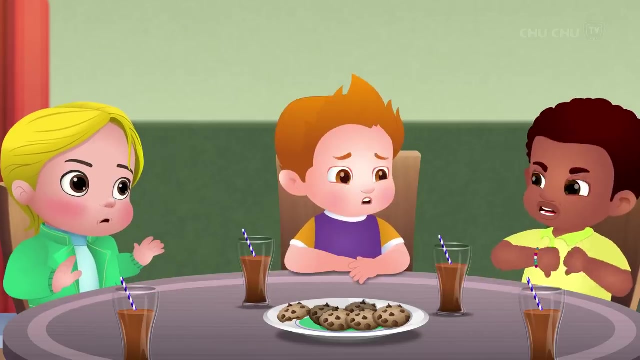 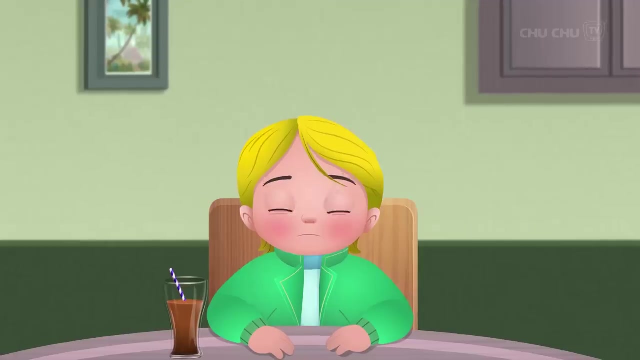 grumbling. This cookie is very hard. This cookie is too soft. My milkshake isn't milky. My milkshake needs more chocolate. Huh, Custly was very disappointed to see his friends fussing and grumbling so much. All Custly.